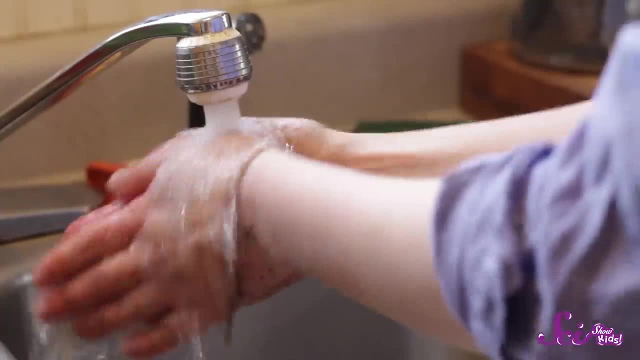 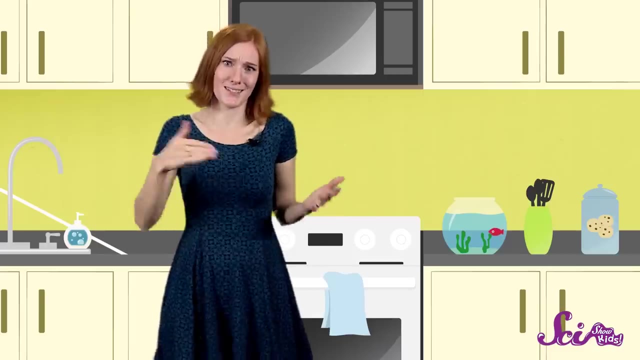 One, the force of the water pushes the mud off of your hands. And two, the water dissolves some of the stuff that makes up the mud. It washes it down the drain. Cool, right, But what about baths? Before we can dive into that, 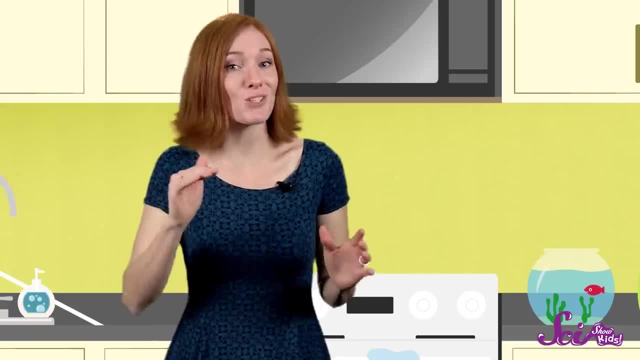 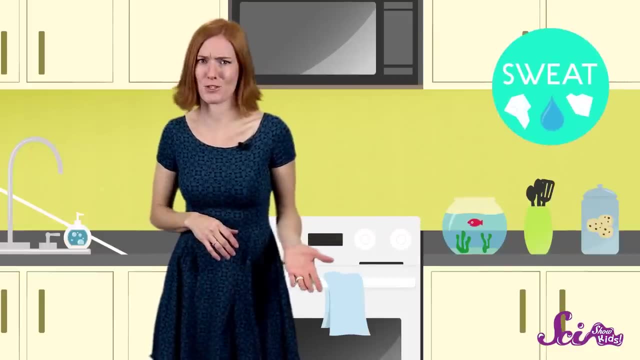 let's take a quick look at how we get dirty. in the first place, Your skin makes its own oil. This natural oil helps your skin stay soft and healthy, And your skin also makes sweat, which we've talked about before too. Sweat is mostly. 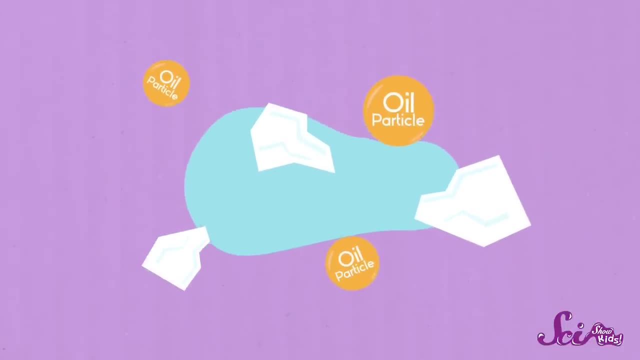 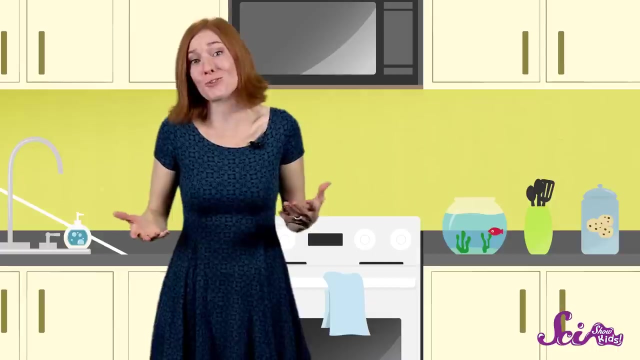 salt and water. When the water in your sweat dries up it helps cool your body down, But it leaves that salt and other stuff behind. So all during the day dirt and dust sticks to the salt and oil. If you let the dirt and 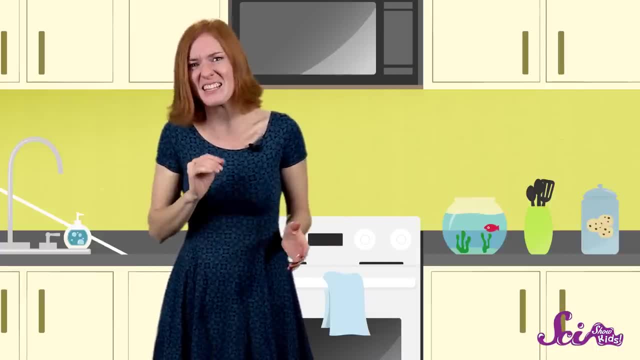 oil build up for too long, it becomes a good place for bacteria and other very tiny living things. So it's a good idea to wash often. Now, when you get in the tub, the water dissolves the salt and a lot of the dirt that gets stuck. 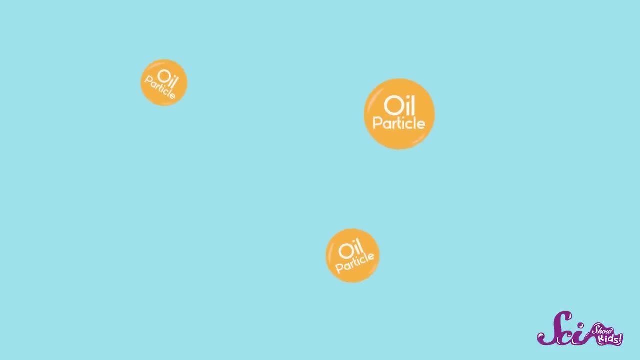 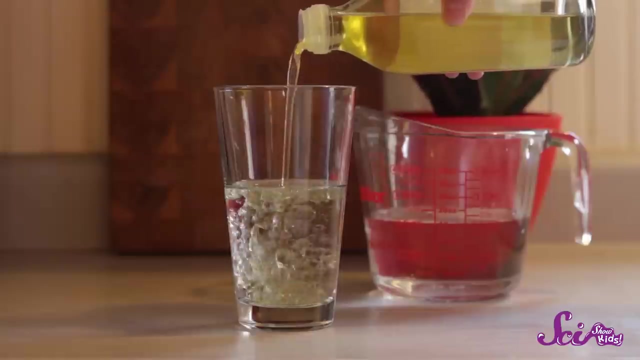 onto your skin. But one thing water can't dissolve is the oil itself. Why? Because oil and water just don't mix. You can see so for yourself. If you pour some water in a glass and add a bit of cooking oil, you'll see that they form two completely. 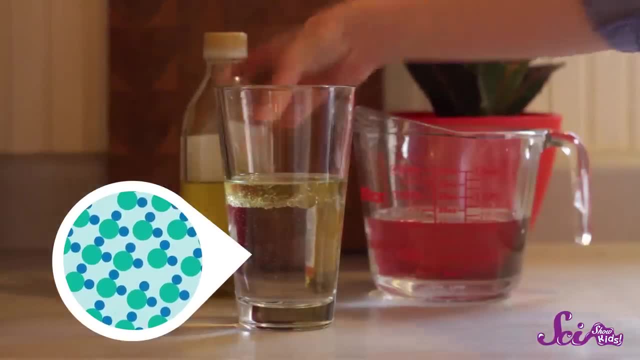 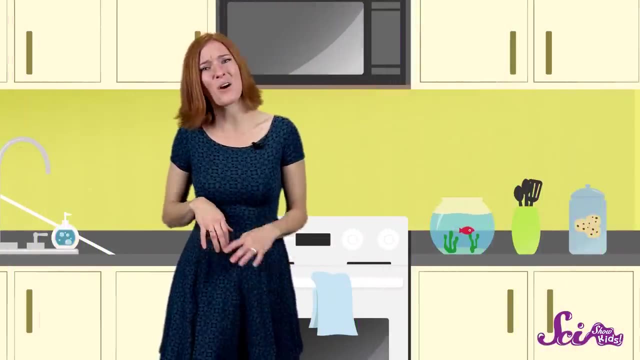 different layers. Water particles are small and stick together very tightly, But oil particles are bigger and don't stick together as well. So if water can't mix with oil to wash it away, then how can you get that oil off your skin? That's where soap comes to the rescue. 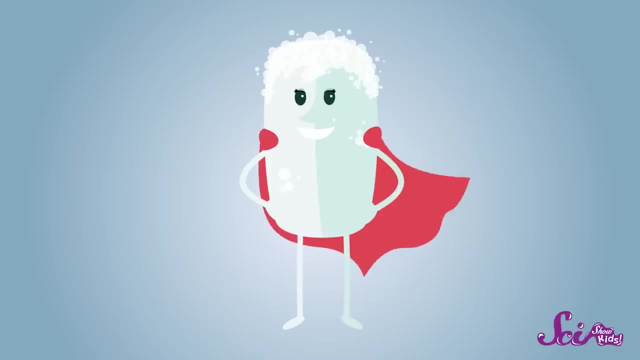 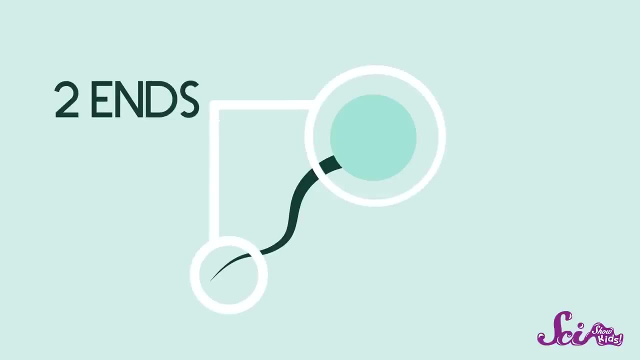 Soap can't dissolve oil, but it can stick to it really well and help wash it away. If you could look at the particles that make up soap, you could see that they each have two different ends And each end is attracted to or pulled toward different kinds of things. 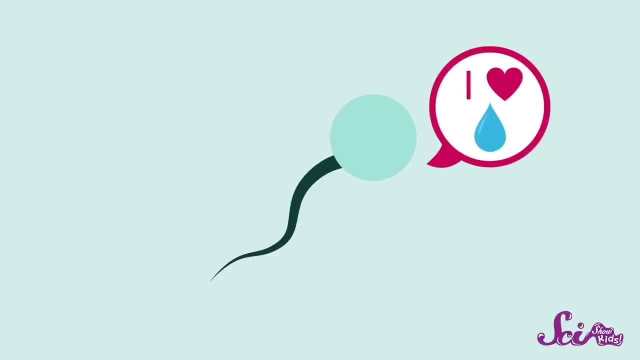 One end of the soap particle is pulled toward water and the other is pulled toward oil. So when you mix soap with oil and water, one side of each little soap particle sticks to the oil while the other side sticks to the water, And then, when you rinse off the soap, oil and water all go away. 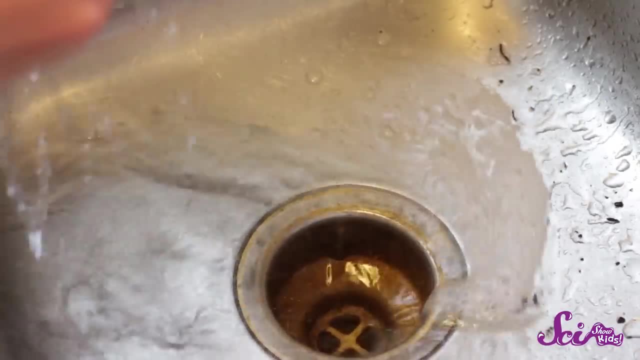 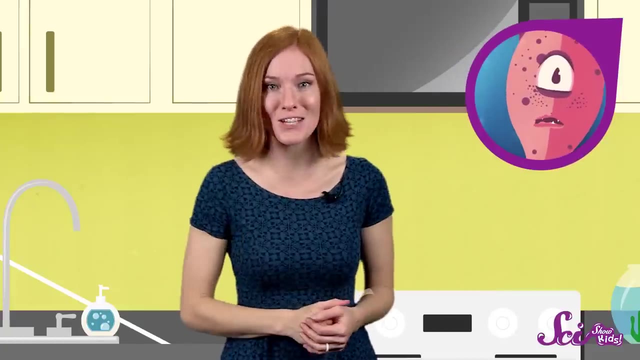 And that's where soap comes to the rescue. So now you know how water and soap work together to get a squeaky clean in the tub. And if you happen to see squid before I do, tell them yourself. Thanks for asking all these great questions. Do you have a question that you would like? 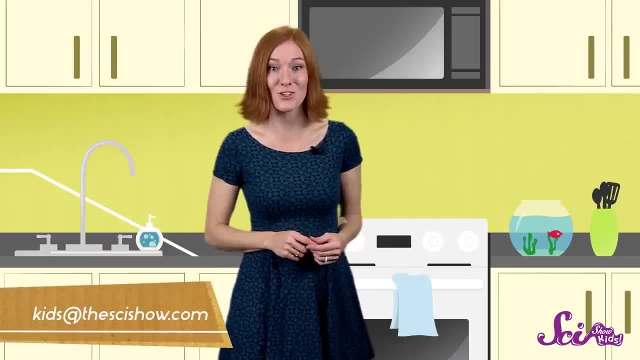 us to answer. If you do, just let us know by sending us an email at kids at the scishow dot com. Thanks, guys, and see you next time.